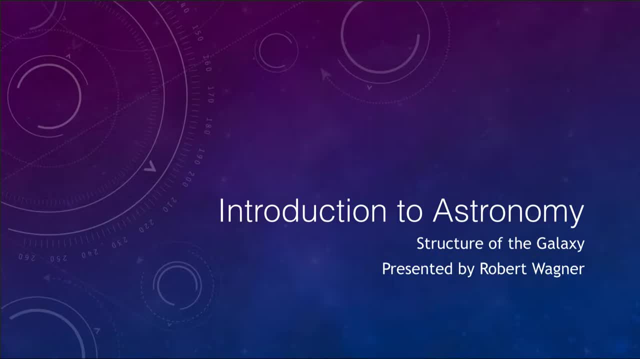 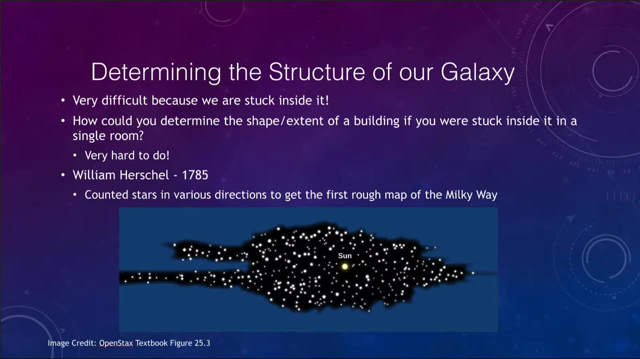 Let's go ahead and get started here, and what we see is, first of all, how do we determine the structure of our galaxy? It's not an easy thing to do, primarily because we are stuck inside our galaxy, So it's a little harder to determine. that then it is. if we could look. 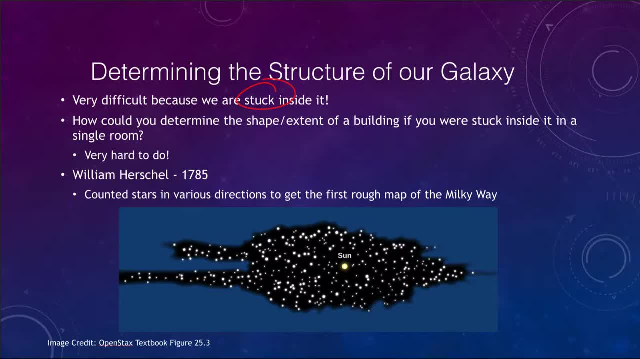 at a different distant galaxy. So an example would be: it would be very hard. how do you know the shape or extent of a building if you're stuck inside a single room? You might have windows to look out to give you some idea, but if you could not move from that room and had not seen the building before, you would have a very difficult time determining how many floors the building has. How high up does it go? How far down does it go? 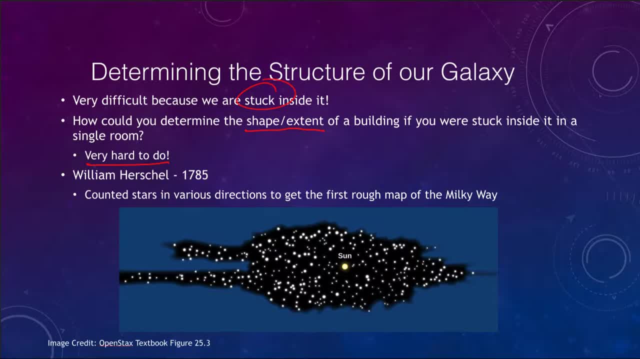 We have a very similar issue with our galaxy. We cannot easily see through our galaxy, And in fact one astronomer, William Herschel, in 1785, counted stars in various directions to try to get the first rough map of the Milky Way, And here what he found was our sun relatively close to the center of the galaxy. 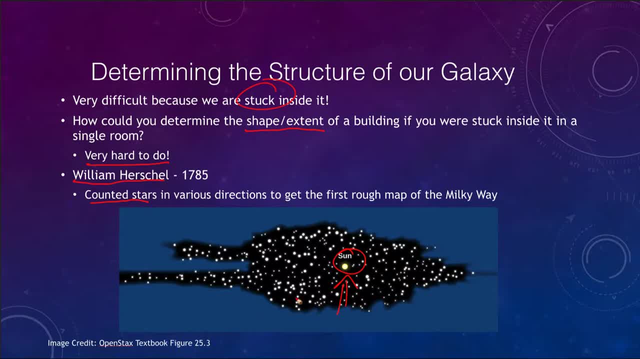 But he did notice that the galaxy was flattened, that there were far more stars in this galaxy, In this direction, than there were in the up and down direction. So he saw that there were far more stars here. Now, one of the problems that he had is that he did not understand that there was a lot of dust. We did not realize that there was dust And in fact, looking off this way would be the center of our galaxy And most of the stars there are completely blocked by the dust. So there are actually a lot more stars here and our galaxy extends a lot farther off here to the left. 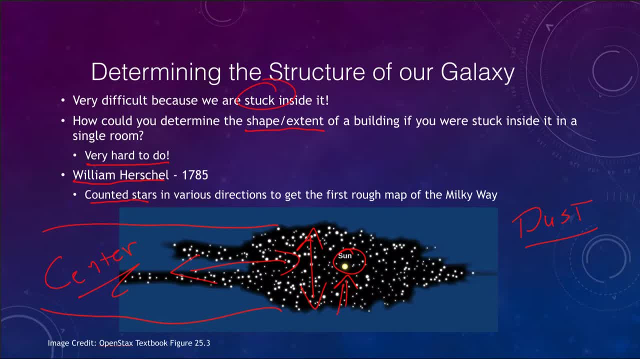 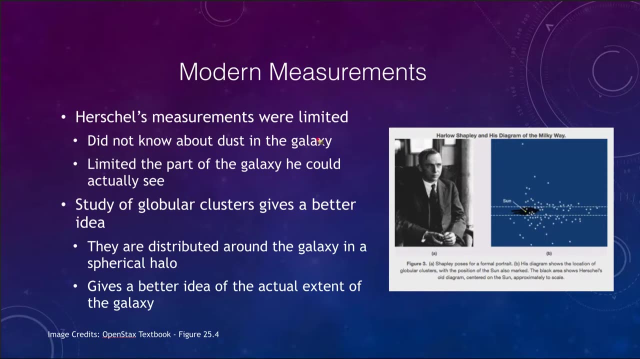 Then it does to the right And while it was a first great map of the Milky Way, it did not tell us the true extent of the Milky Way galaxy. So more modern measurements because, as I've said, Herschel's measurements were limited, meaning that he did not know about dust and that limited the part of the galaxy that he actually was able to view. 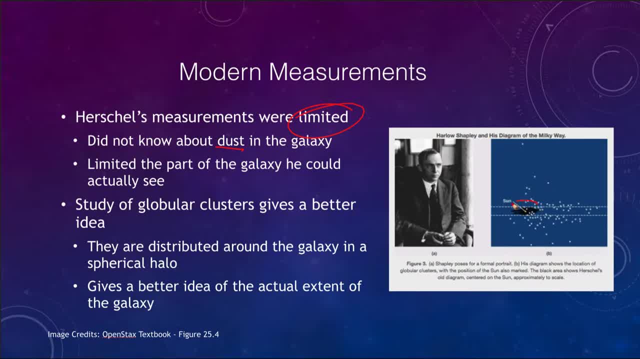 So, as we see in the image here, Herschel's image is just this little black section here. He was only looking at a very small part of our galaxy. However, looking at the globular clusters gives us a better idea. That's because they are distributed pretty much uniformly around the galaxy in a spherical halo, and this tells us a much better idea of what 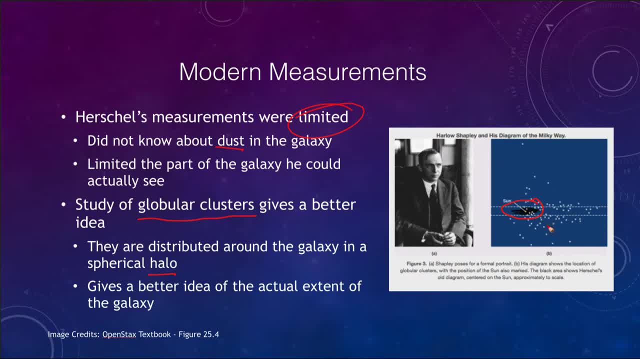 the galaxy is like. So we can see that the galaxy is. now. we have all of these dots in here. each of these little dots represents a galaxy, But you really understand exactly who it is: This huge, beautiful galaxy, This really amazing galaxy. And now, as you can see, it is also measuring just a much more balanced but discoverable connection between different galaxies. And so, since all subjects are soño-spkiego cors assassins, this galaxy tends to find others, rather Cristobal meyers, and so we're going to learn a few more steps. 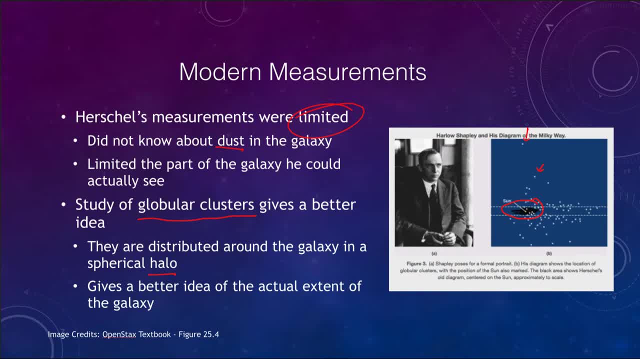 globular cluster. They can be seen over large distances, So we can see them even when they are very far away, And if we can assume that they are pretty much centered on the center of our galaxy, then that means that the center of our galaxy 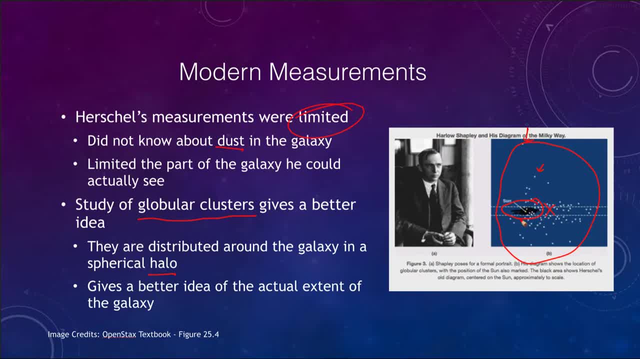 is here, roughly well outside even the little section that Herschel was able to observe back in the 1700s, So studying these globular clusters and Harlow Shapley here was one who was able to do that And he was able to find that. no, we're. 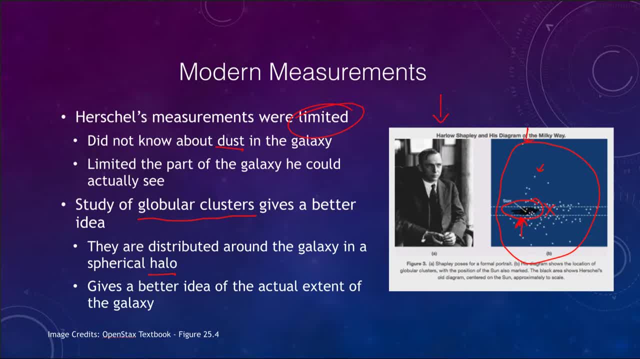 not near the center of our galaxy, as Herschel had found from his measurements, but we are actually well away from it. So let's look at what our galaxy is made up and what our galaxy is composed of, So the different components of our galaxy. 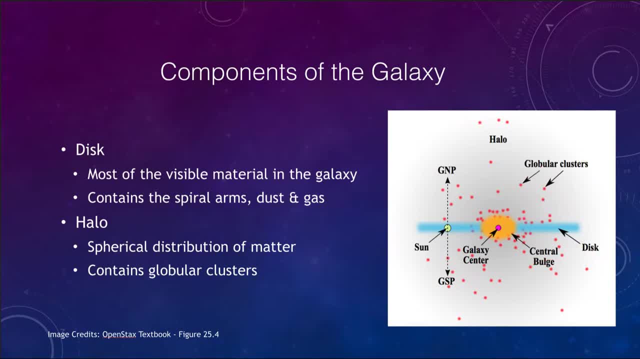 we have several different ones here And what we have is we have the disk of the galaxy, which is really most of the visible material. When you look at a spiral galaxy, which is what our Milky Way is, most of that material is the disk material. 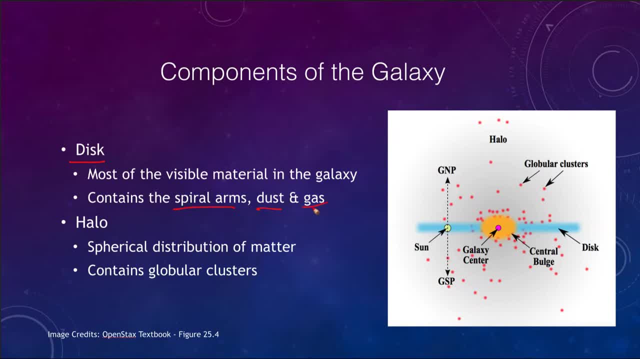 It contains things like the spiral arms and the dust and the gas and is where stars would be forming. So it would be sites of star formation And that also makes it very easy. It would be visible because there are bright stars forming there. So our disk shown down here is the very flattened area. 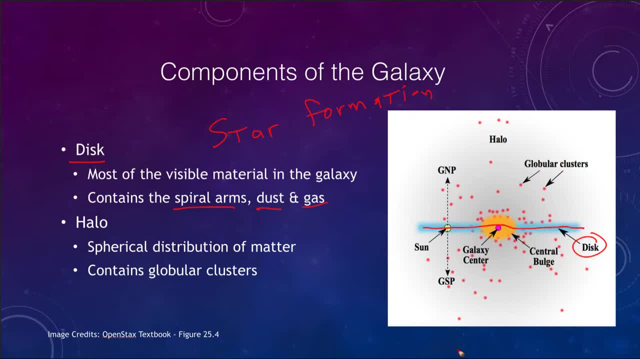 that goes right through the central portions of our galaxy and is where the galaxy is flattened. Now there's also the halo, which is a spherical distribution. That's where those globular clusters that Harlow Shapley saw were And when he measured those, those globular clusters? 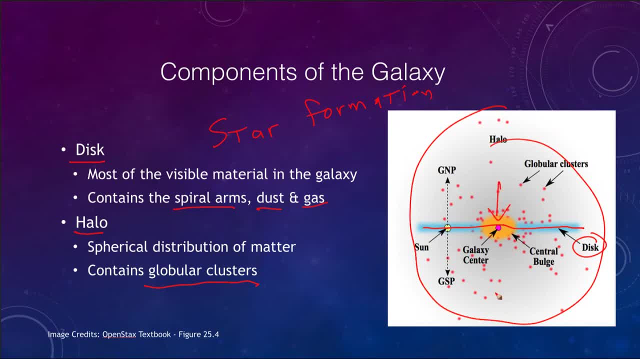 are then centered on the Milky Way. So we happen to be located here, actually towards the outskirts of the galaxy, But there is a halo, a lot less material. It has the globular clusters, but has a lot less material, a lot less. certainly not any gas and dust, that. 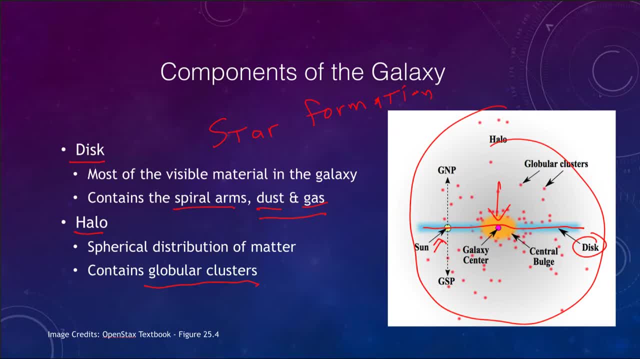 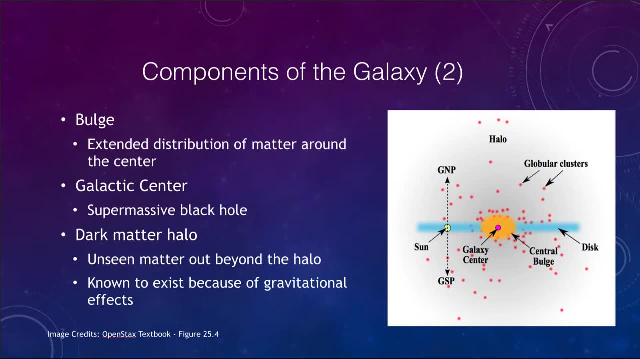 would be forming new stars. Now there's a couple other components as well And we have the bulge of the galaxy. So the central bulge is noted here. That is an area That is kind of in between the disk and the halo. 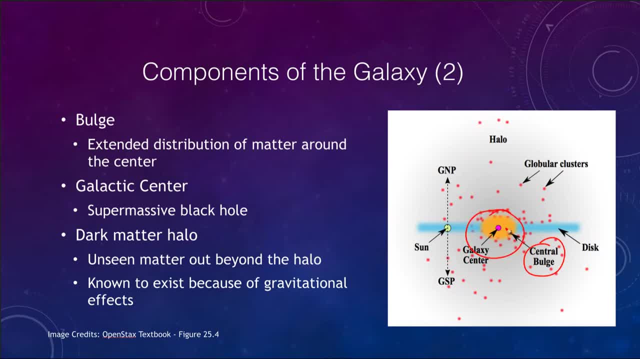 The disk is very flattened, The bulge is extended a little bit And then the halo is a big spherical area around it. So this is an extended distribution of material around the center of our galaxy. The galactic center itself contains a supermassive black hole, about four million solar masses. 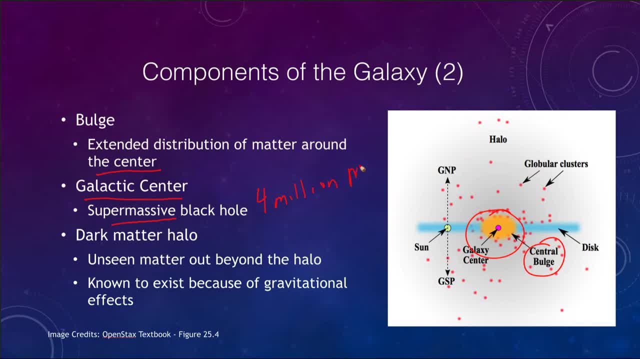 So four million times the mass of our sun. And then out beyond that not shown in the image, is a dark matter, halo. Now we saw the halo itself. That's stuff we can see, But there is also much more unseen or dark matter. 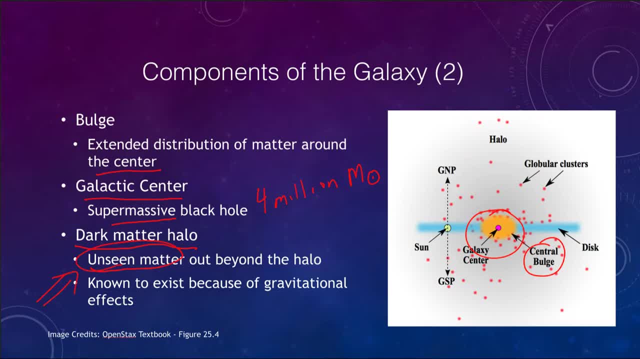 around the halo. This is very important. We know that it exists because of gravitational effects And we'll take a look at that later- But we know that it exists there, that there must be far more mass than we can possibly see And dark matter. 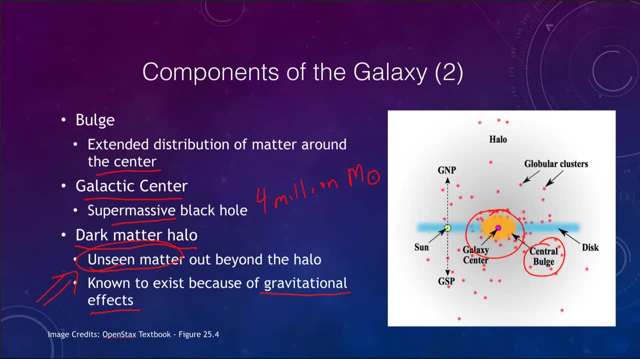 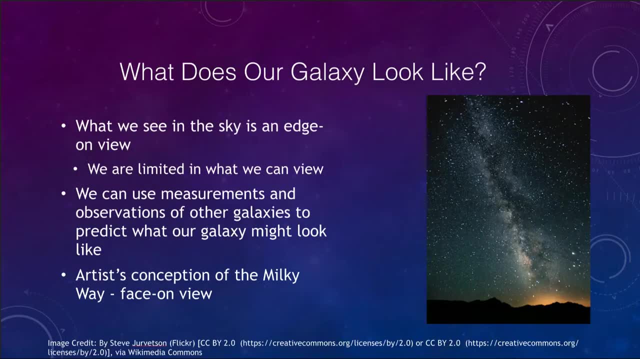 is one of those things that astronomers are continuing to study today. So what does our galaxy look like? Well, what we'll see is that our galaxy, when we look at it, we actually see an edge on view. So we do not see our galaxy as a great spiral galaxy. 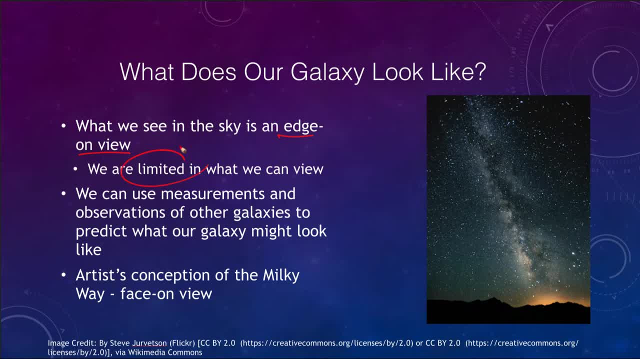 We see it edge on because we're sitting inside it, And it gives us a very limited view of what we're able to see. We can use measurements and observations of other galaxies, however, to kind of predict what our galaxy might look like. 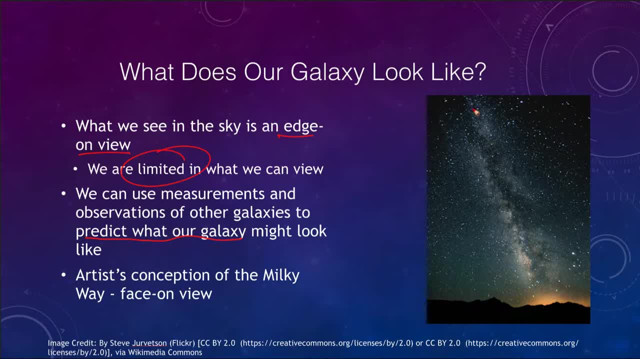 So we can make some measurements: figure out where different dust clouds are, figure out the extent of our galaxy, where the denser portions are, where the least dense portions are, and use that to be able to try to determine what our galaxy might look like. 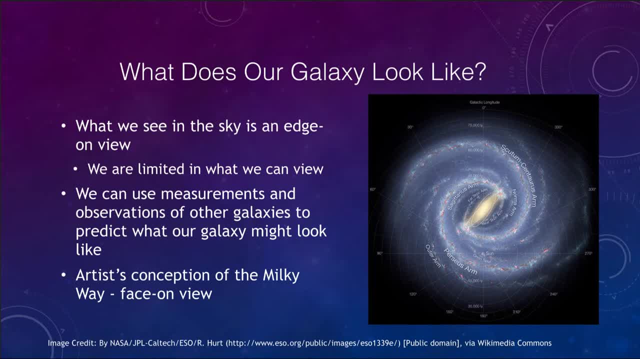 And an artist's conception might give us something like this, that we would then be able to see our galaxy. So here is the central bulge of the galaxy, in towards the center. The whole thing we're seeing is the disk. We get the distinct spiral arms spiraling out from the center. 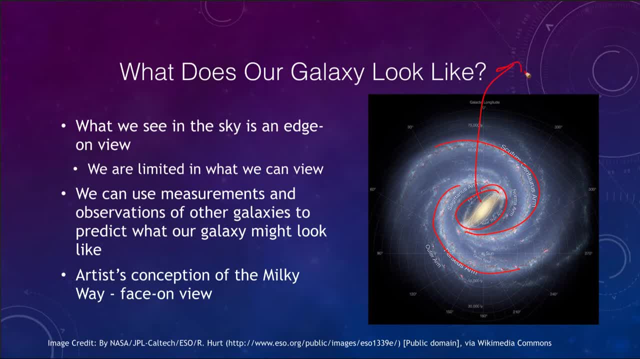 And we also. in our case, we see a central bar. That means there is a bar of material going through the middle of the galaxy, And that is important because we see a number of other galaxies that have it. We have this as well. 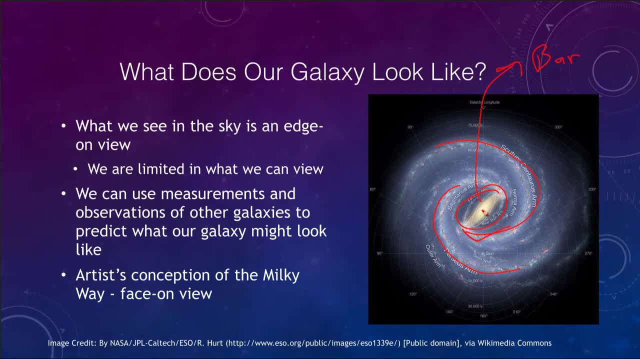 And in fact, the spiral arms start from the edge of the bar, not from the actual center of the galaxy itself. So this is an example of what we might be able to see if we could travel 100,000 light years away, or 10,000 light years away, straight up out of our galaxy. 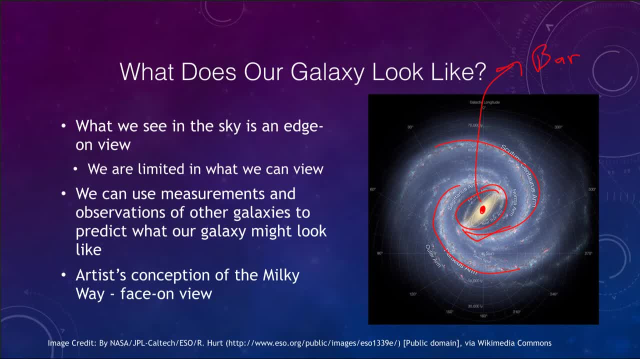 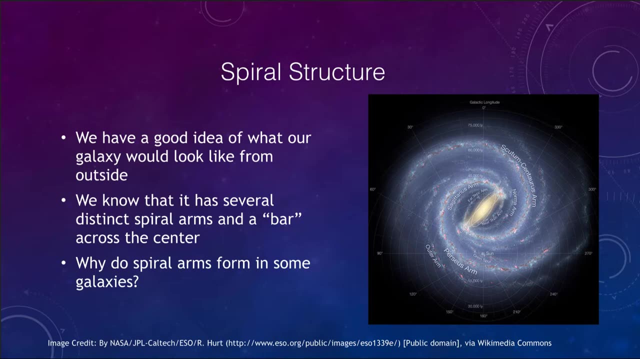 and look back down on it to get that full view of our galaxy. So what do we see when we see the spiral structure? Well, we see some of it in the image here We can take a look. What do we know? We now know what our galaxy looks like a little bit better. 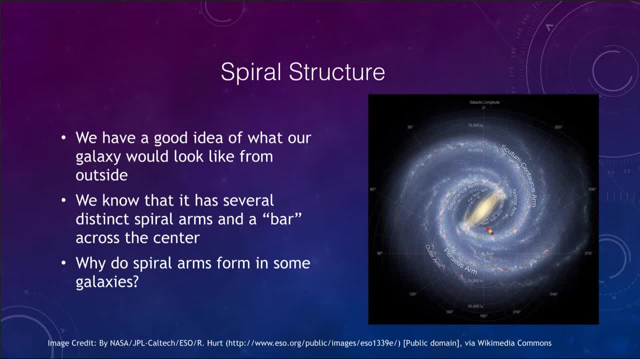 We see that there is very distinct spiral structure. As I showed before, we have various different arms. There's the Sagittarius arm into the Perseus arm out here And the Scutum Centaurus arm is the main arms, But there's also some other ones going here. 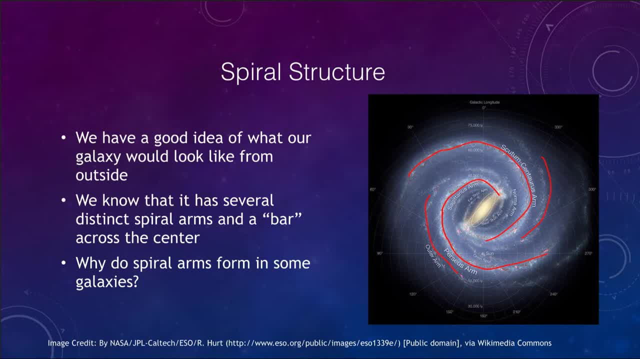 So our galaxy doesn't have just one or two spiral arms but has a number of them that have formed. We know it has those several distinct arms and the bar going through its center which, again, we've seen those in some galaxies. And a question can be: why do we get spiral arms in some galaxies? 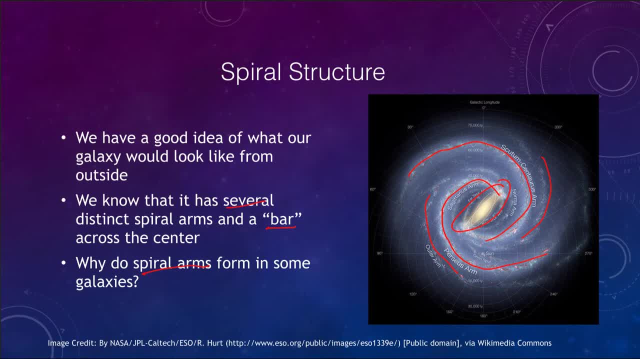 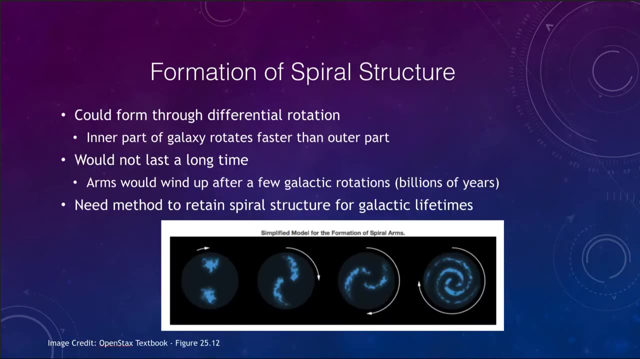 but not all of them. So why do certain galaxies show us a spiral arms And what we think in terms of how spiral structure forms? we can actually look at that Very briefly here And what we find is that how do spiral arms form? 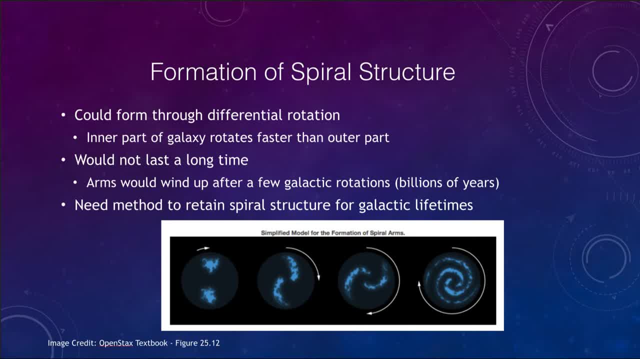 Well, one thought is that maybe they form because the galaxies undergo differential rotation. Now, that's not unusual. It simply means that the inner part of the galaxy rotates faster than the outer part. So you could imagine that if you had blobs of material that 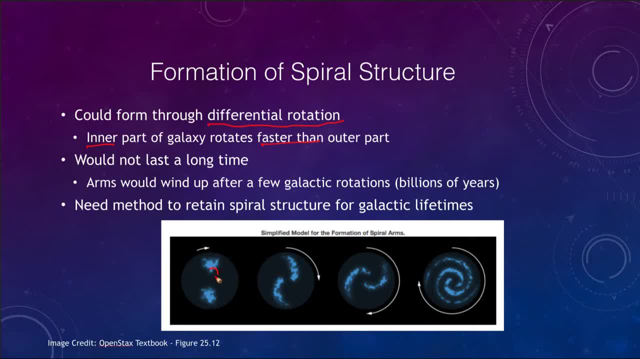 stretched across the galaxy, with the inner parts rotating faster and the outer parts rotating much slower that they would spread out over time. So you'd start to get them spread out a little bit here and more here, And then finally you would form distinct spiral arms. 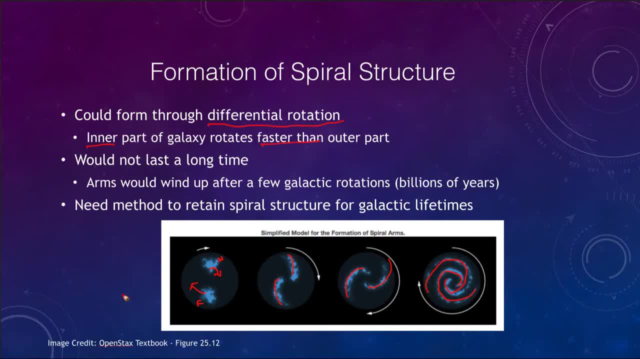 just like we saw in the estimation of what our galaxy might look like. The problem is, these would not last a very long time. After just a few galactic rotations, which might only be a billion years or so, they would wind up and be completely gone. 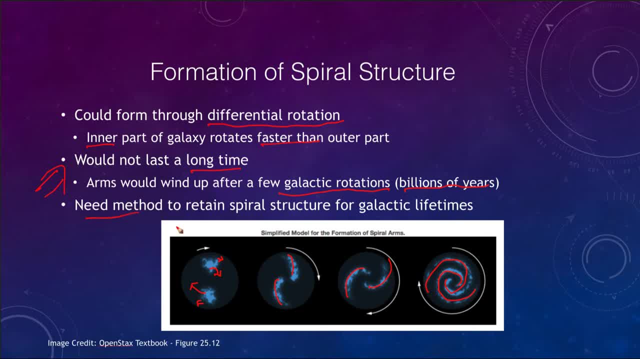 So, while it can form spiral arms, we need some method to be able to retain the spiral structure for the lifetime of a galaxy- And we are talking 10 billion years in that case, since we see spiral galaxies at various ages And the way we believe this works. 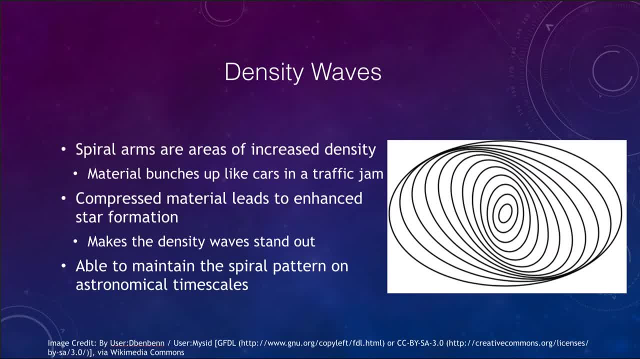 is through what are called density waves, So a spiral density wave. what they are is areas of increased density, much like the way material bunches up, the way cars bunch up in a traffic jam, So the compressed material as the density wave travels. 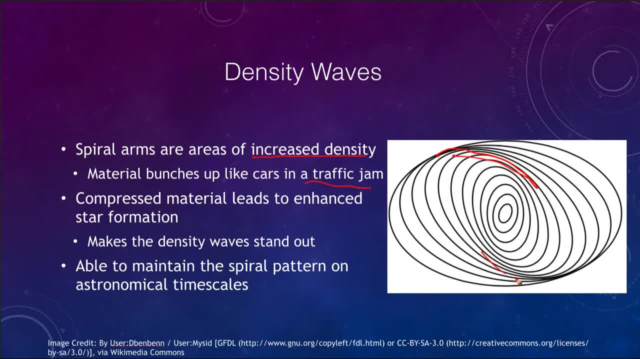 through where that compressed material is, here and here, then that forms. that is where star formation is going to form. So stars are going to begin to form in these areas where the material is compressed. You push more material Together. you're more likely to begin to be able to form stars. 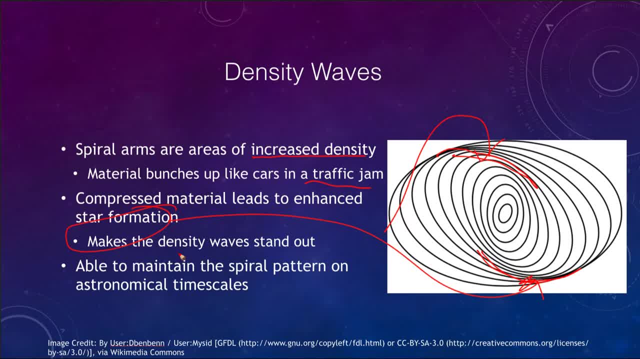 So, while the density waves themselves would be invisible, this highlighted star formation makes the density waves stand out and gives us the pattern Now, because the density wave would move much slower than the actual rotation of the galaxy. this would allow spiral pattern to maintain. 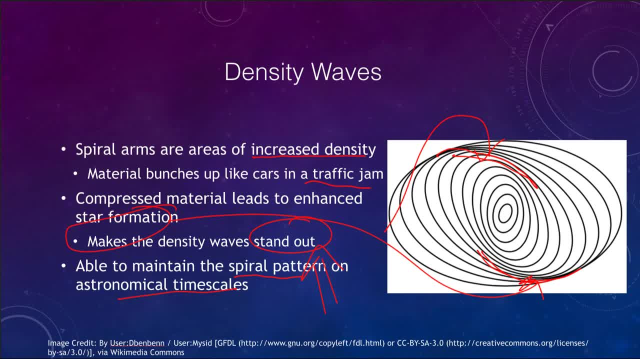 for astronomical time scales. So, just as a traffic jam, The density wave itself can move slower than the individual cars. If there are cars bunched up on the highway and you're moving through that, you slow down as you're moving through it and then you pick up your speed again.